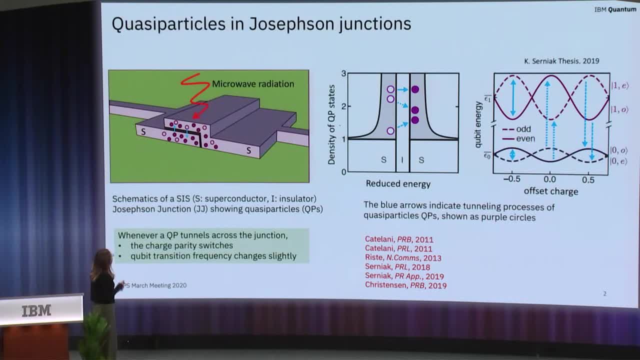 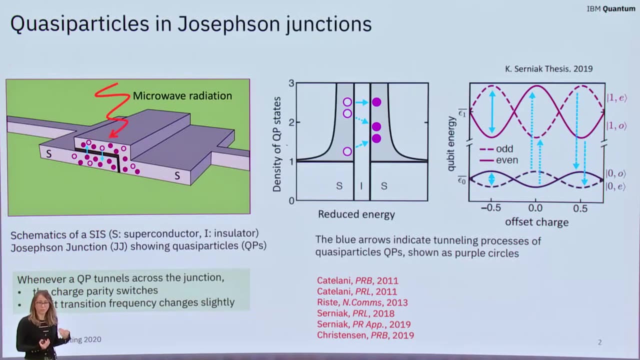 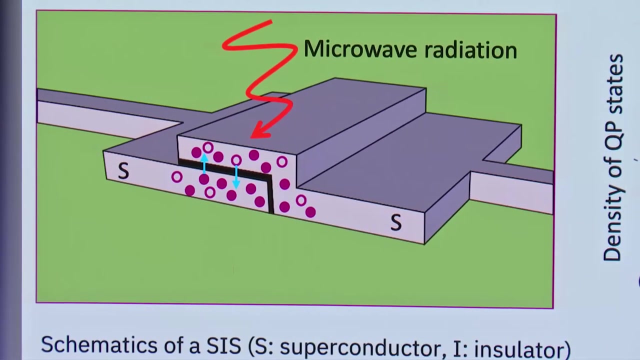 constitutes the barrier. Such a structure at finite temperatures can accommodate electron and hole-like excitations out of superconducting ground state. Mainly we call them quasiparticles. When we apply microwave radiation to those junctions, quasiparticles directly couple to the electromagnetic modes of the qubits and 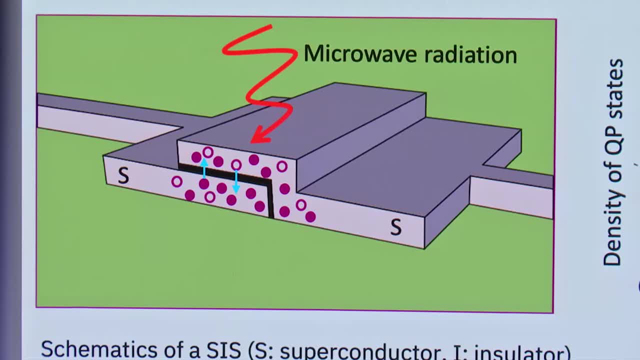 possibly limit the coherence of our devices. When a quasiparticle tunnels across the junction, it can cause the qubit to move in the opposite direction of the qubit. When a quasiparticle tunnels across the junction, it can cause the qubit to move in the opposite direction of the qubit. 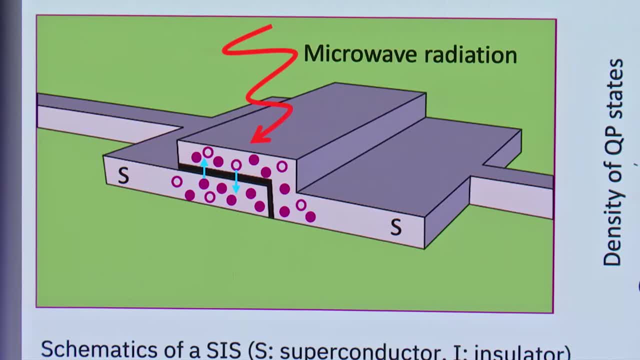 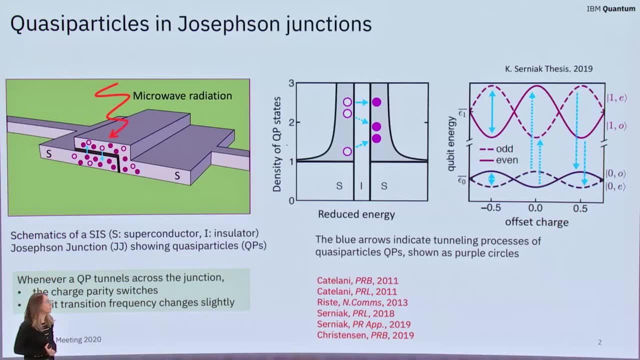 When a quasiparticle tunnels across the junction, it can cause the qubit to move in the opposite direction of the qubit On the otherside of the junction. that's the bás más kurz term. after all, a quasiparticle tunneling across the junction is a linear. 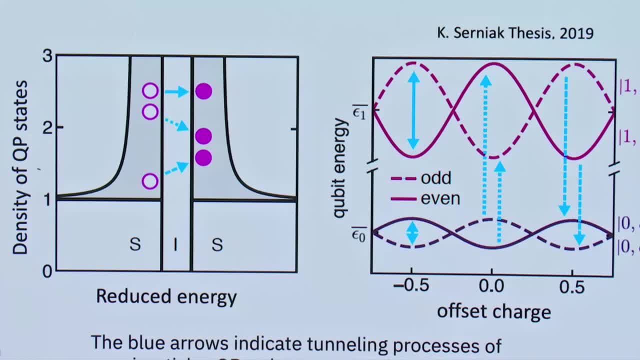 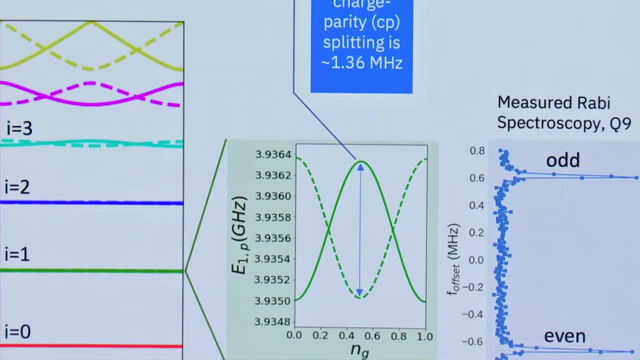 ��iniál norm On the Antonov-R questionnaire. it's basically the same measure to be bought And those quasi-particle events can manifest themselves as transitions between the charge parity manifolds in the energy spectrum of a qubit. You can see it on the far right. 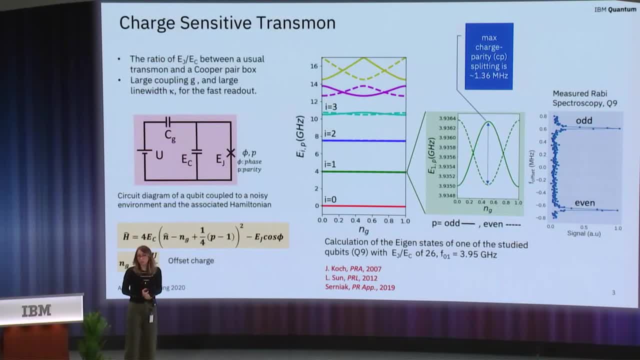 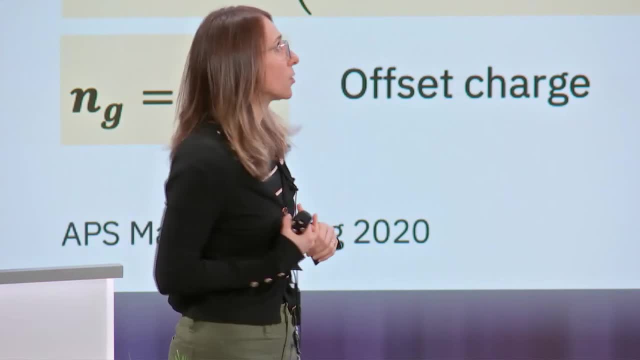 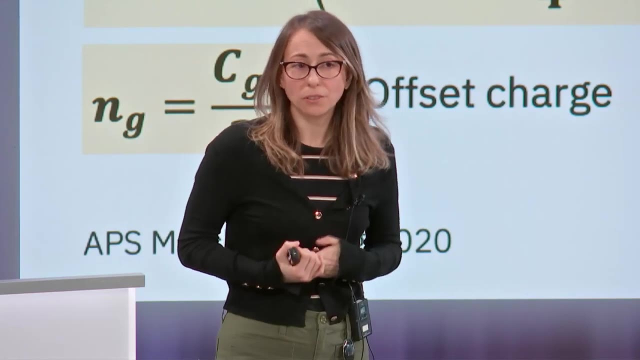 So the question is: what type of qubit do we need for these measurements? At IBM, we focus on transbound qubits. However, at the extreme transbound regime, where EJ is significantly larger than EC, the qubit transition frequencies are insensitive to the charge fluctuations. 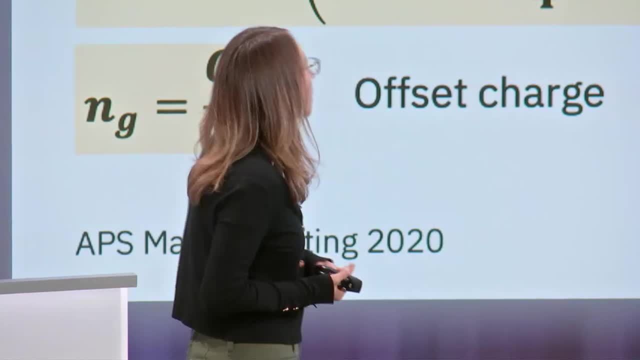 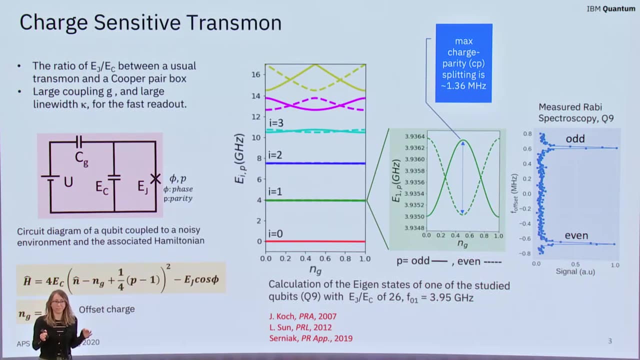 In a different scenario, where EC is comparable to EJ, the dispersion in the energy levels are so overwhelming, so it also makes the detection of the tunneling equally difficult for us. So what we need is a qubit operating at an intermediate regime, with a moderate EJ to EC ratio. 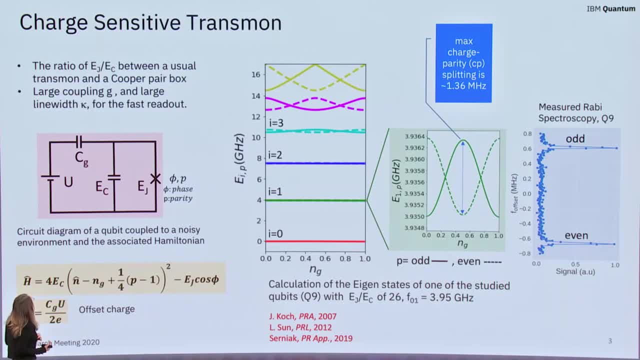 In addition to this requirement, we also need large transbound qubits. We need large coupling G and large line-knit kappa for fast readout. By using the simple circuit model and associated Hamiltonian, we can calculate the eigenstates of a qubit as a function of NG, which is the offset charge. 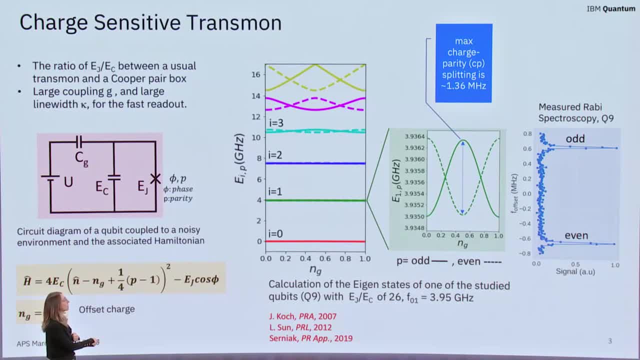 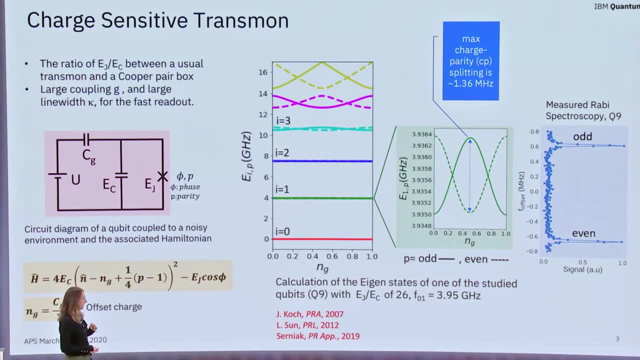 and we index those things according to plasmonic states And these calculations are based on an EJ to EC ratio of 26, and we use some other parameters belonging to a qubit we experimentally studied- I think it was Q9.. 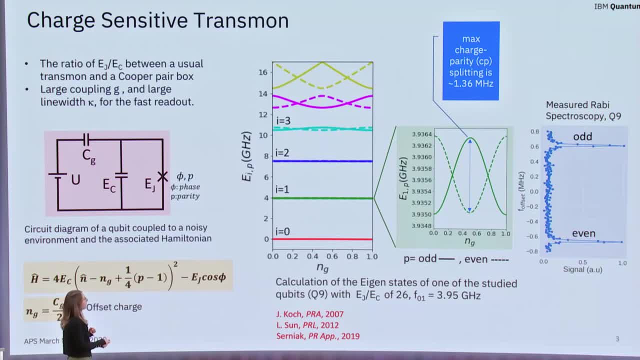 So when we focus on the first excited state of this calculation, we see it's not a flat bend. In fact there are two charge manifolds which are corresponding to different parity states, So we can calculate the splitting maximum splitting from here. 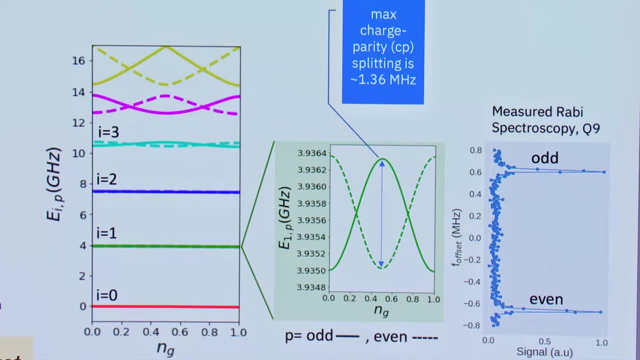 which is 1.36 megahertz, and we can directly see the splitting from an experimental state which we can essentially take in Revit spectroscopy on the far-right. And these symmetrical peaks correspond to odd and even parity states, which is direct proof of presence of those parities. 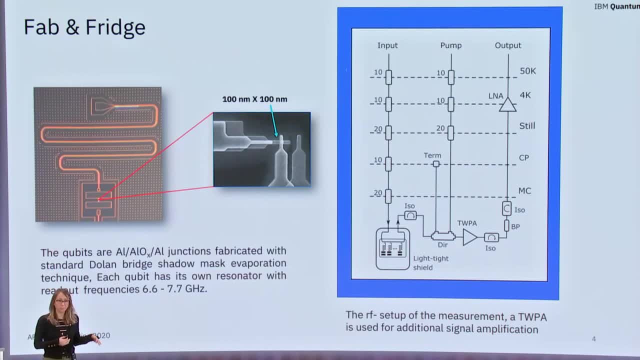 Our qubits are basically aluminum, Aluminium oxide-aluminum junctions fabricated with standard Dolan breech technique, And the junctions are shunted by very large nylon reels. niobium capacitors which are connected to niobium resonators. 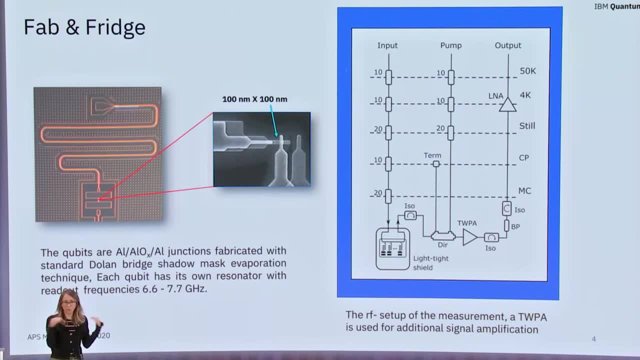 And individual niobium resonators are coupled to a common transmission line. And on the right you see the RF setup of our measurements. As you can see, the input line is heavily attenuated to be able to protect the qubit from excess radiation. 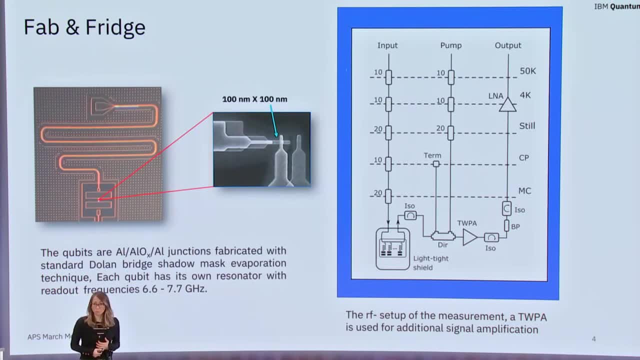 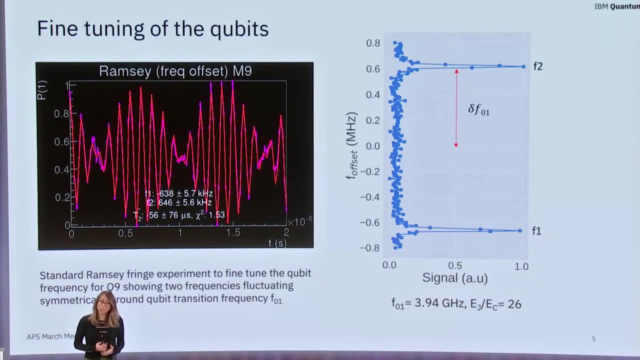 And we also use the TUPA as a quantum limited amplifier to be able to improve the signal to noise ratio. So, prior to the Ramsey experiments sensitive to the time scale of the quasi-particle tunneling measurements, we did some standard spectroscopic measurements to be able to obtain the readout. 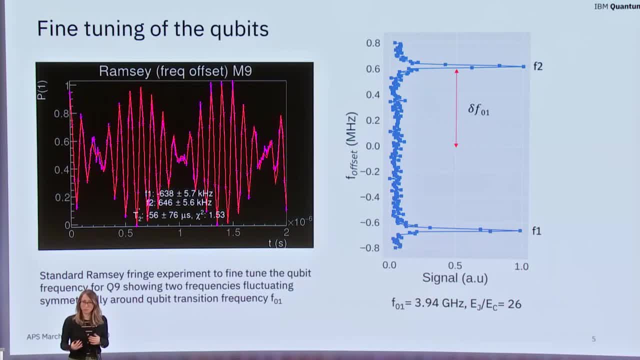 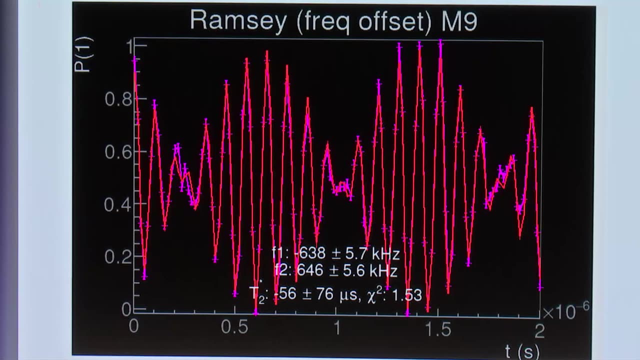 mode resonances and the transition frequencies for the qubits just roughly. And then actually to be able to fine-tune the qubits, we performed standard Ramsey experiments. Here you are seeing one example here. In this Ramsey experiment we were able to fit the oscillations into a sum of two sinusoids. 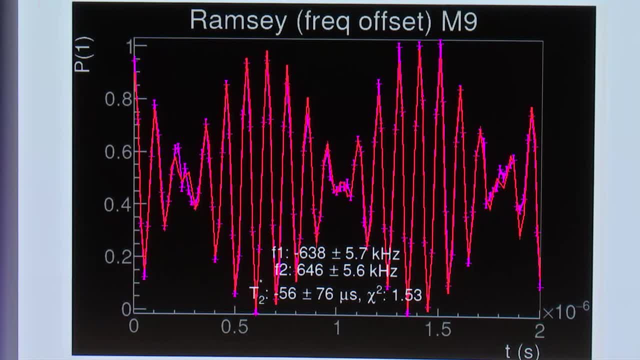 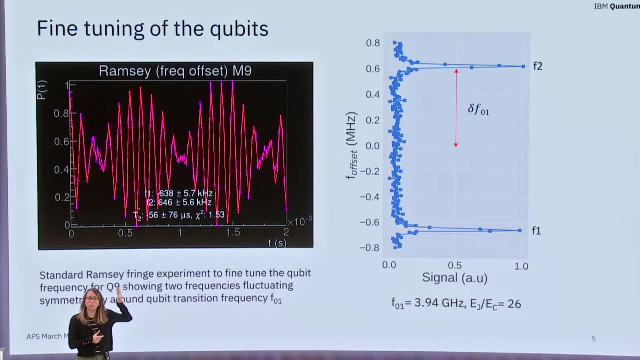 fluctuating symmetrically around F01, which is the transition frequency of the qubit And the Rabi spectroscopy I've shown you before, which was successfully showing the parity space. the peaks are separated by two delta F01.. Delta F01 is the detuning from the F01.. 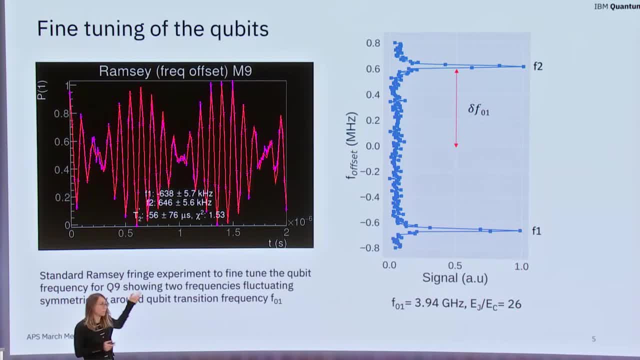 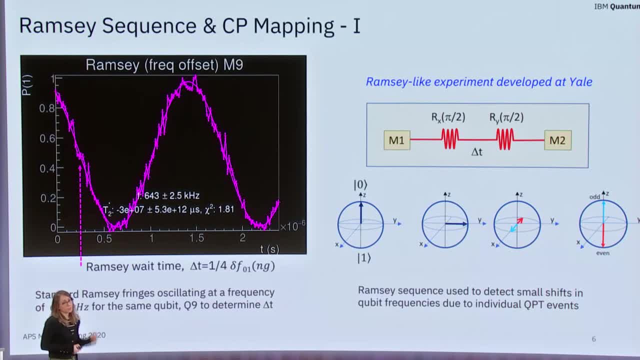 And the delta F01 is the detuning from the F02.. And the delta F01 is the detuning from the F02.. At the end of the spectrum of oscillations you can actually see that it's very high cases, quite a large number of oscillations in a column of light, and that this is how. 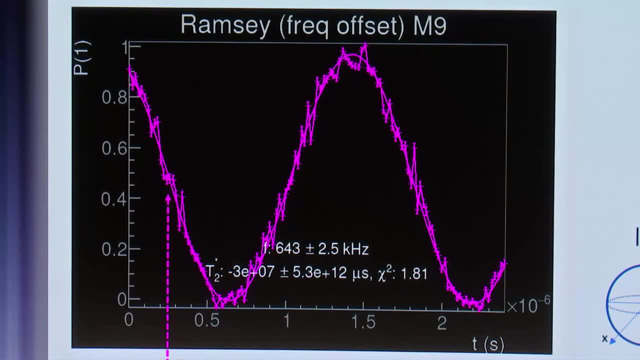 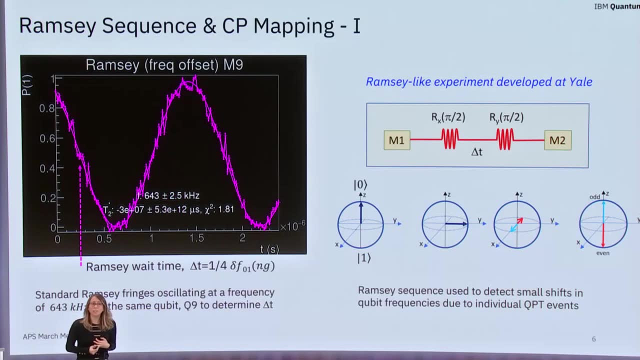 the onzeity linear is responding. So you have the dynamic sexta-galaxial efflu楽ation system for the multiplax distributions For 31 minutes. It can also have aRAW effect, So this light display will tell you how many clearly visually visible basal��x chirals. 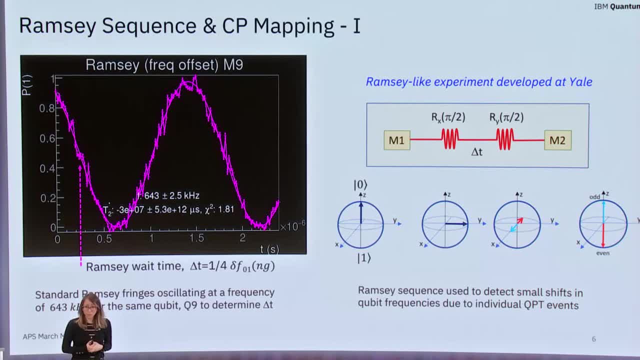 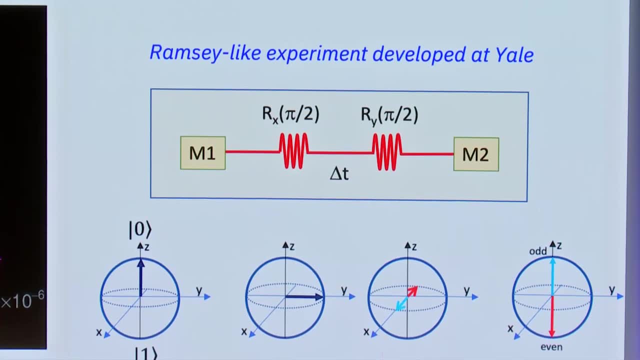 appear. The experiment starts with an application of a pi over 2 pulse around the x-axis. That brings the qubit on the equator of the Bloch sphere here, And then the qubit picks up a plus, minus pi over 2 phase. 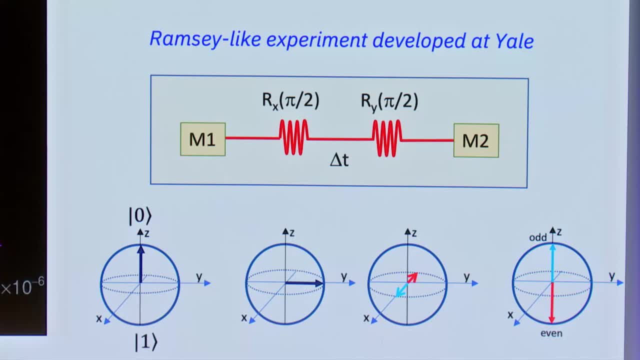 depending on the charge parity during an idle time. So that brings the different parities on the opposite side of the equator of the Bloch sphere. Then a second pi over 2 pulse is applied around the y-axis to be able to map the parity to the charge. 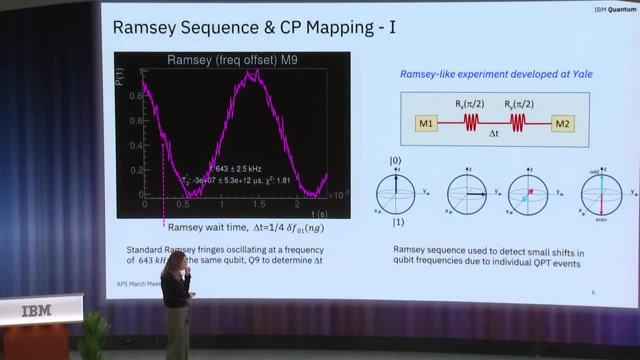 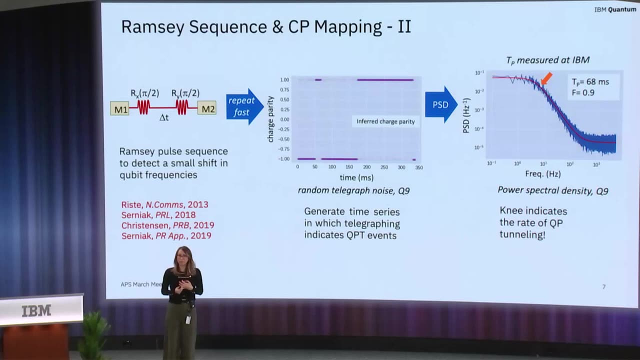 basis state. So basically, if the parity is odd, the qubit ends up in the excited state. If the parity is even, qubit goes back to the ground state. So to be able to observe the quasiparticle tunneling events, 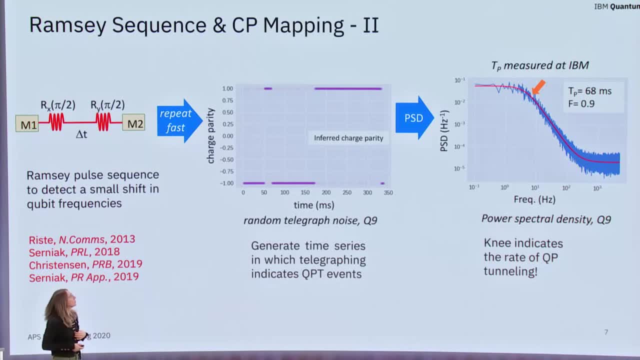 in real time. we repeated those CP mapping in every 100 times. We read it in microseconds for a second. Then the power spectral density of those fluctuations are averaged over 20 traces. Finally, we fit the power spectral density into a characteristic Lorentzian of random telegraph nodes. 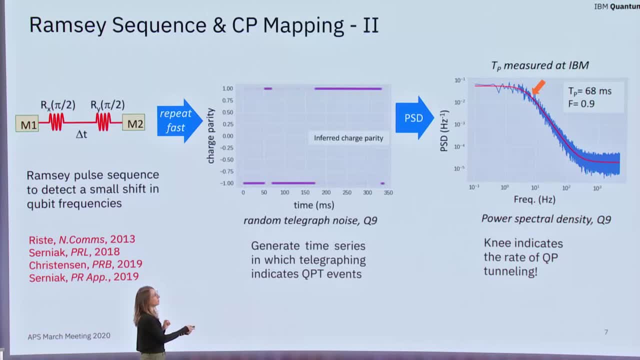 From there we were able to get some values really important to us, like the switching time, TP and the fidelity of the measurements. So these measurements are obtained and then they're transferred to the next wave, then the third wave at the IBM labs, giving us extremely long. 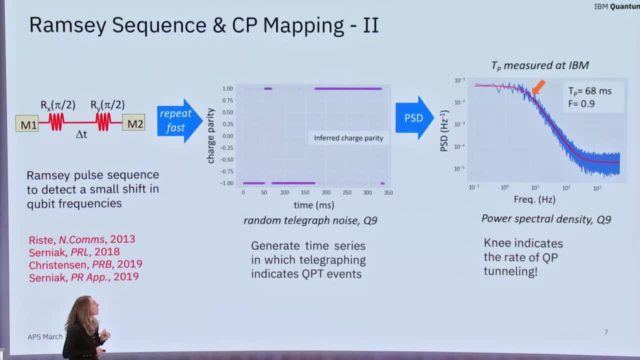 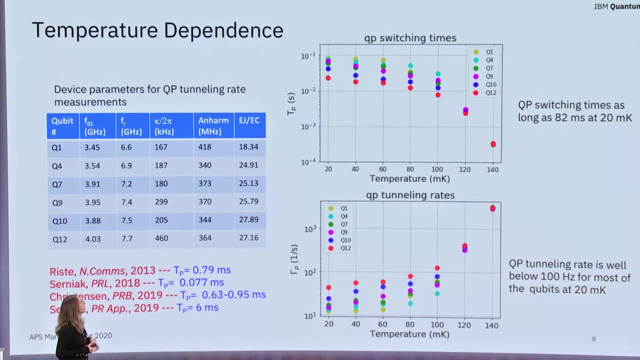 quasiparticle switching times with a very high fidelity To be able to see the impact of the quasiparticle tunneling events on coherence. we looked at the switching times, thus the quasiparticle tunneling rates, along with T1 and T2 values, as we are changing. 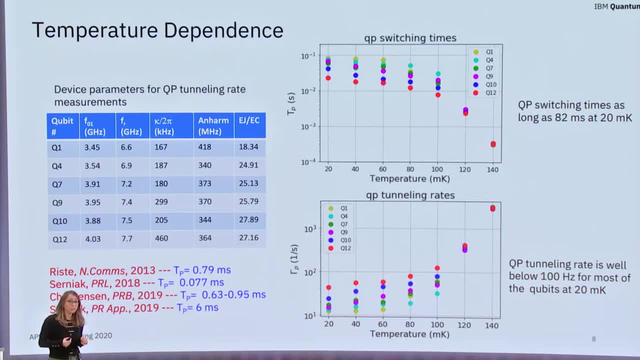 the mixing chamber temperatures. We did it for over 20 qubits and here you are seeing some of the representative qubits. So at low temperatures our switching times were as long as 82 milliseconds, which corresponds to only 12 quasiparticle tunneling events per second. 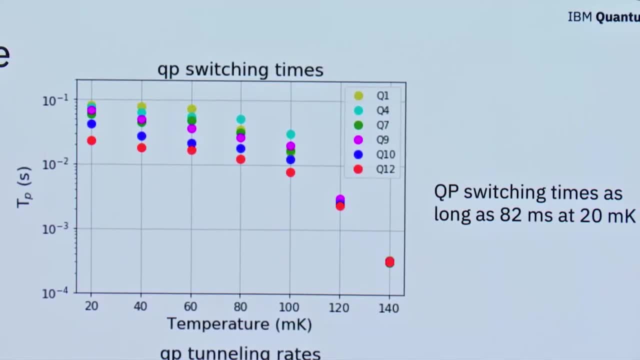 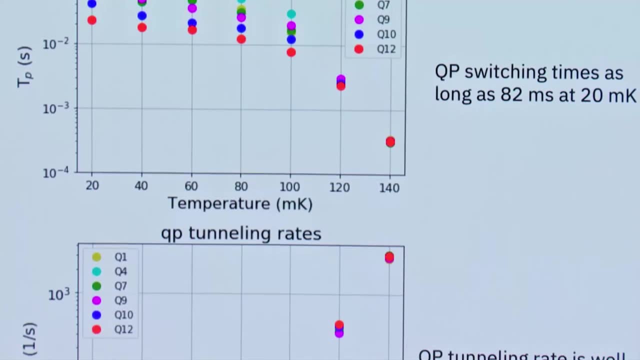 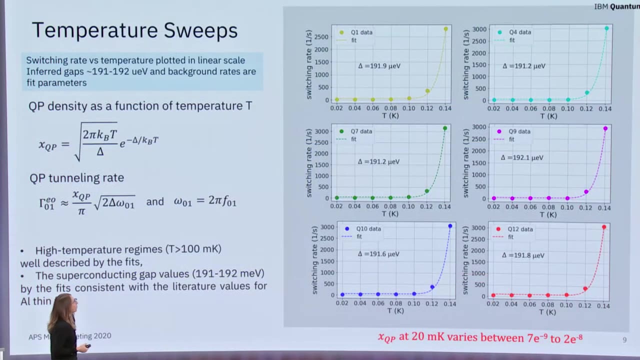 And the rate actually, if you look at the rates here, so beyond 100 millikelvin, they start dramatically to increase. This is very important. Here the switching times T1 and T2 start to drop. Okay, so we modeled the temperature dependence. 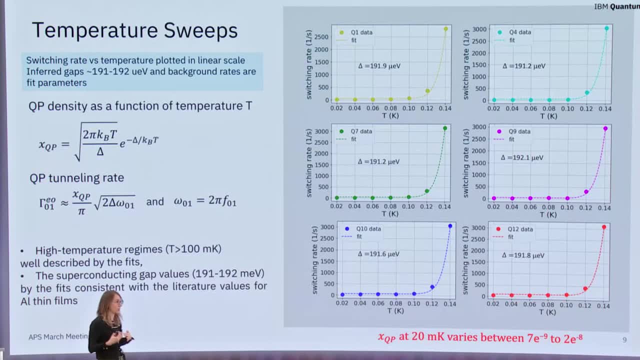 of quasiparticle rates for the same set of junctions. Here you can see the data. So the quasiparticle-induced relaxation rate is linearly scaled with the quasiparticle density, which is the exponential function of superconducting gap. 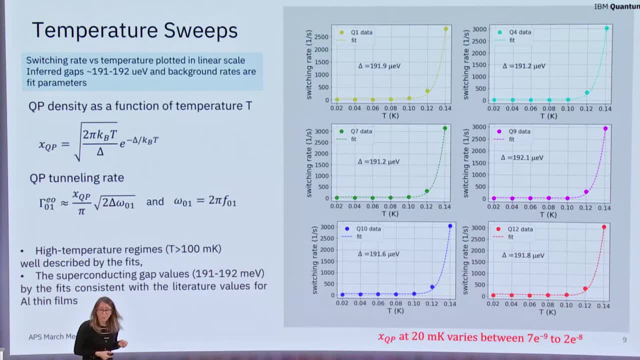 and temperature. We fitted the data plotted here in the linear scale and we have a great agreement at the high-temperature regime for each qubit. The inferred superconducting gap we used as a fit parameter turned out to be 192 microelectron volt. 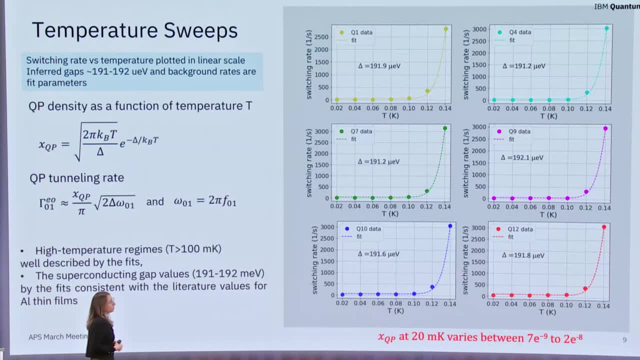 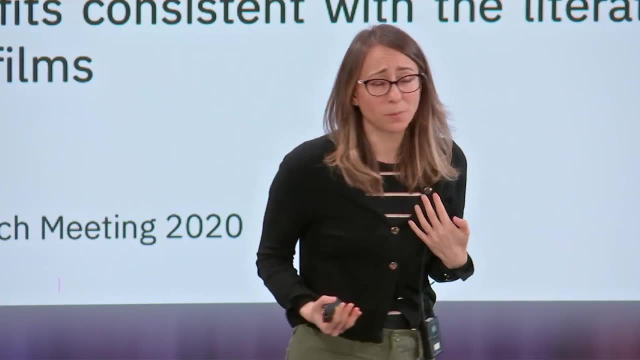 which is very consistent with the literature value of the aluminum tin film. We also estimated the quasiparticle density at low temperatures, which varies between 10 to minus 9 to 10 to minus 8.. I think it's an order of magnitude smaller than the previously. 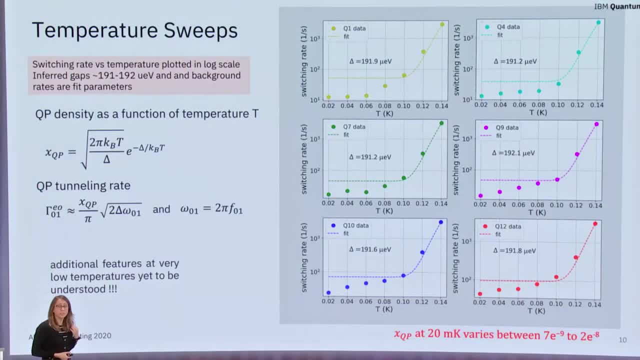 reported measurements. So if you use the same data and plot it in the log scale, you can see the disagreement in the low-temperature regime between data and fits. Although we don't fully understand the reason for this discrepancy, it might be an indicator. 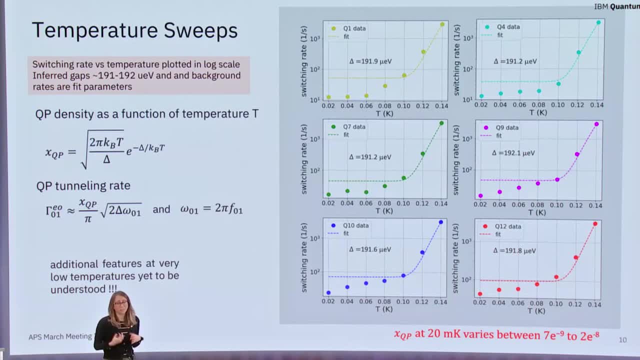 of an interesting physics. Our qubits are a little bit different than the qubits used in similar studies, such as the qubits are controlled and measured in two-dimensional architecture. In addition to that, all our readout resonators or the transmission lines are made of niobium. 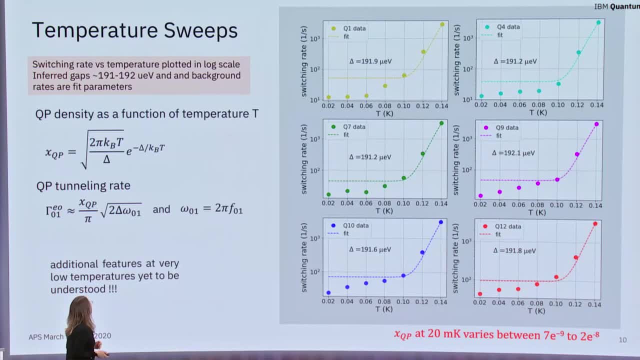 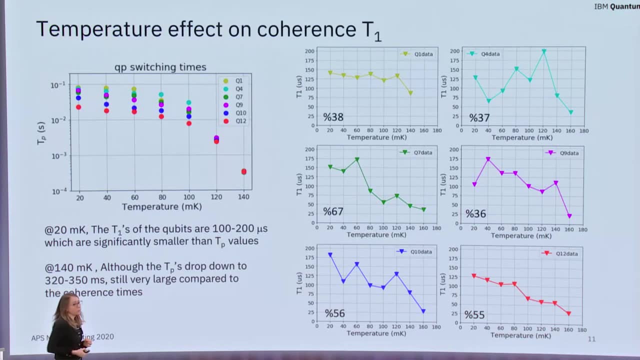 instead of having all circuitry in aluminum. So these are some topics to explore as a future study To be able to get a better understanding of this. we complement the previous data set. We also looked at the temperature dependence of the coherence times T1s. 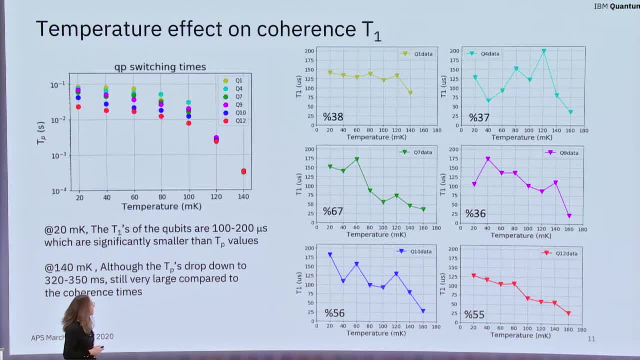 So you can see the data here from the same set of qubits. So at low temperatures we have fairly high T1s, varying between 100 to 200 microseconds. However, they are significantly smaller than the Tp switching time values. 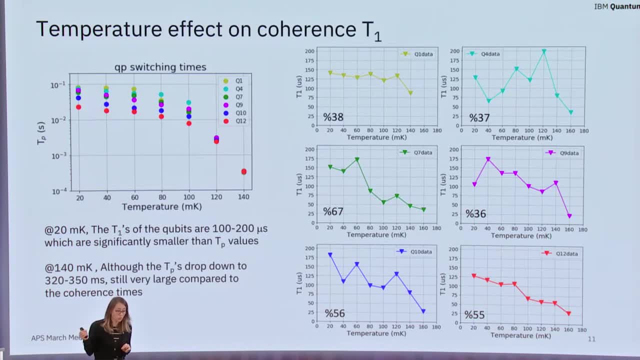 And this fact doesn't change- when we heated the junctions to the elevated temperatures, So beyond 100 millikelvin. despite the dramatic decrease both in T1 and Tp values, they never become comparable, suggesting the coherence in our devices is not limited by the quasiparticle tunneling. 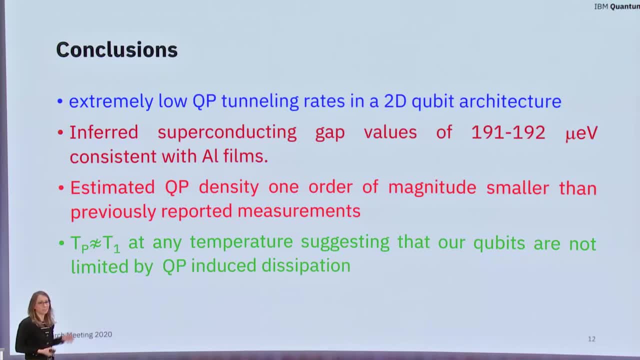 So, in conclusion, we detected extremely long switching times, thus extremely low quasiparticle tunneling rate in two-dimensional architecture. So our inferred superconducting gap values are very consistent with the literature values. The estimated Qp density is one-order magnitude. 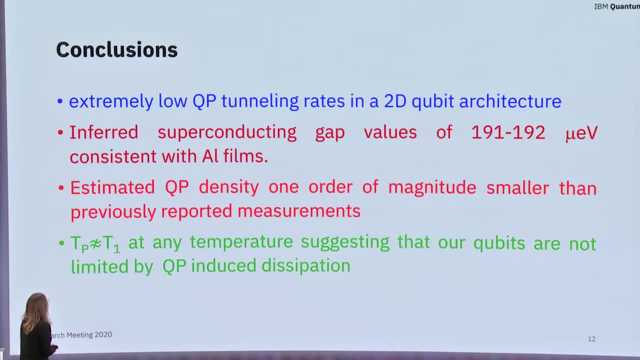 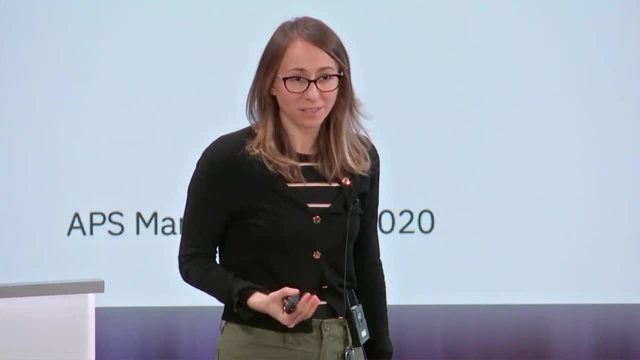 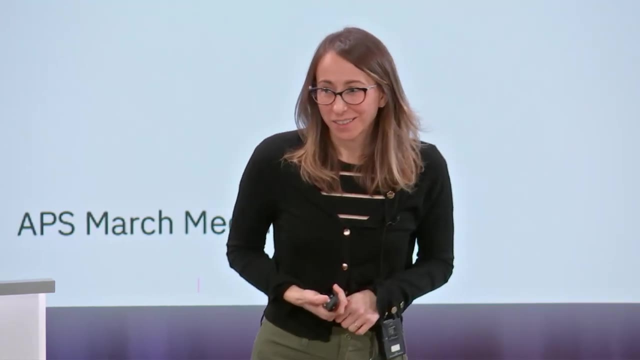 smaller than the reported experiments And the fact that Tp values are much larger than T1 at any temperature, suggesting that our qubits are not limited. the coherence of our junctions are not limited due to quasiparticle tunneling. This is it. Thank you.